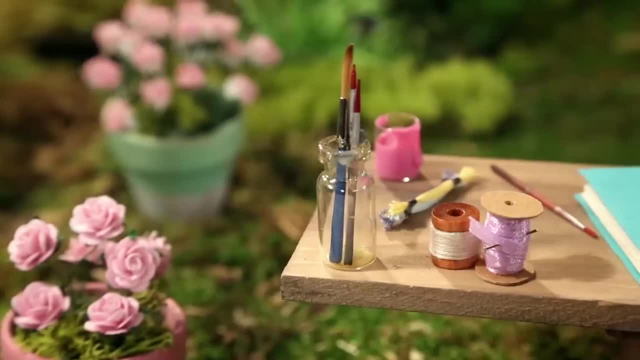 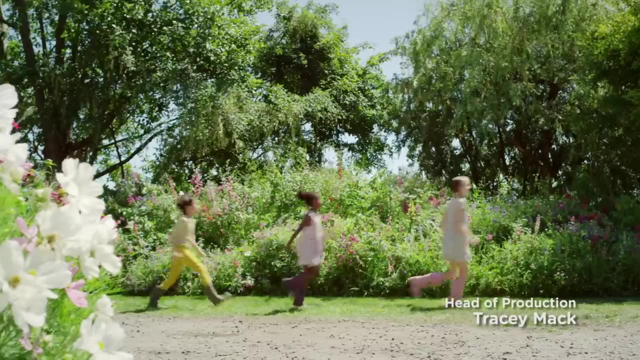 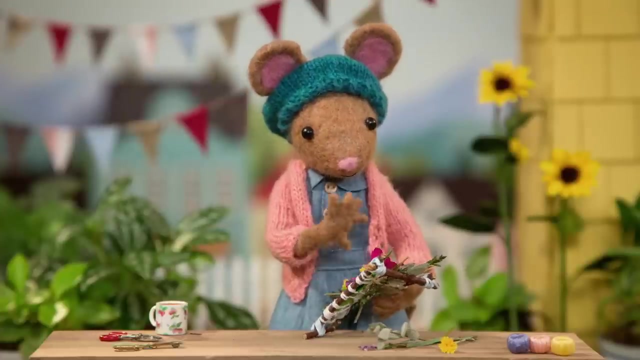 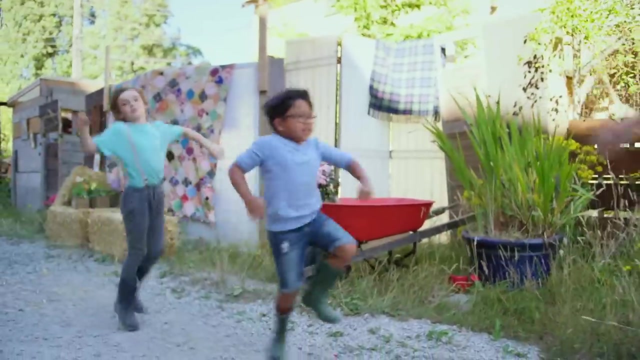 Meet Daisy. She's got a way of making beautiful things. You never know what nature will teach her, what inspiration will bring. D-O-Y, D-O-Y Daisy. what are we making today? D-O-Y, D-O-Y Daisy, I bet we'll make something great. 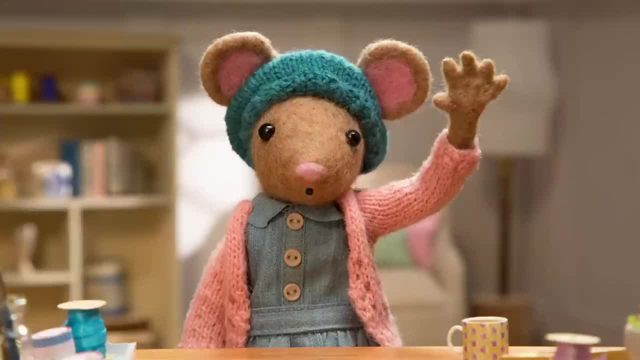 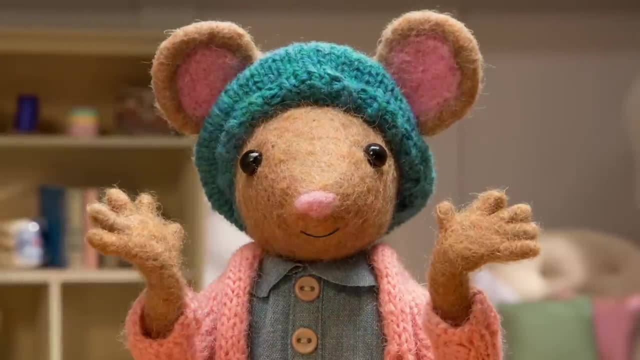 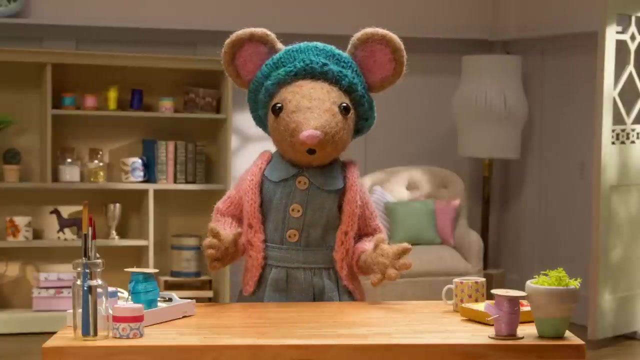 Hello Gumboot Kids. Hi Daisy, Do you hear that It's a thunder and lightning storm? Wow, I love it when it's stormy out and I'm cozy inside my studio. Would you like to make a thunder and lightning storm inspired nature craft with me, Gumboot Kids? 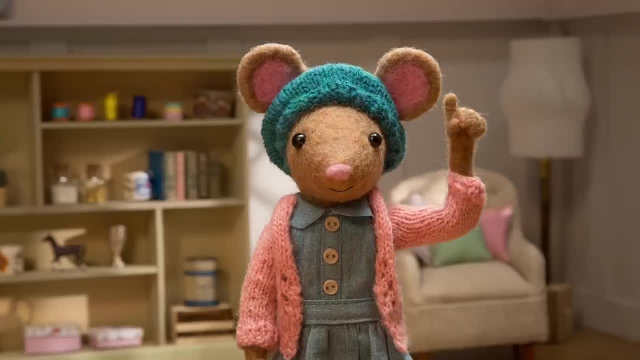 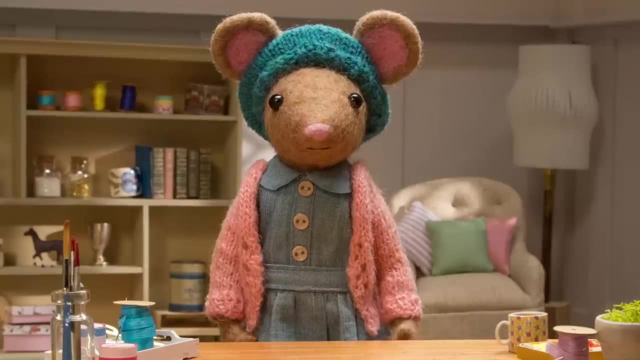 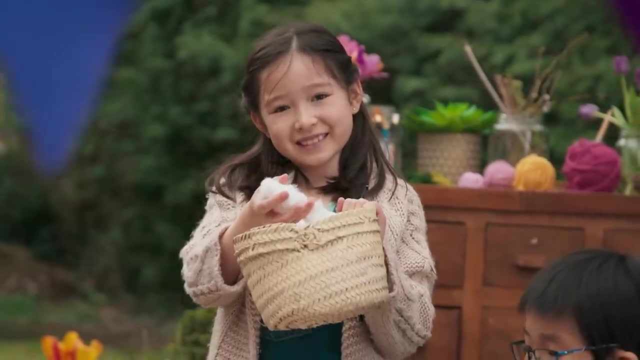 Yay, Okay, step one: Let's make a storm cloud. Cut a paper plate in half, Then use a hole punch and make six holes along the flat edge. That's it. Then glue on some cotton balls to make your cloud. 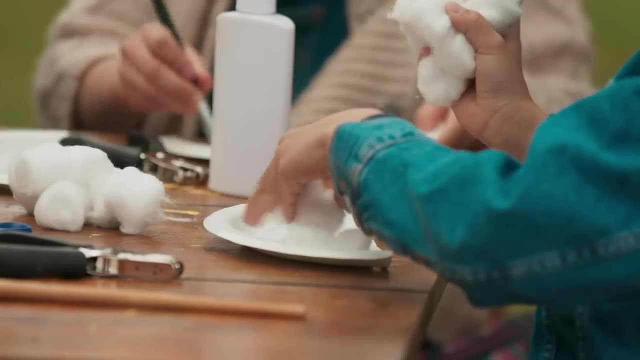 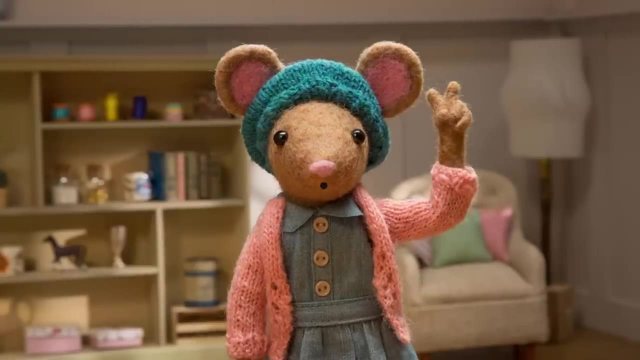 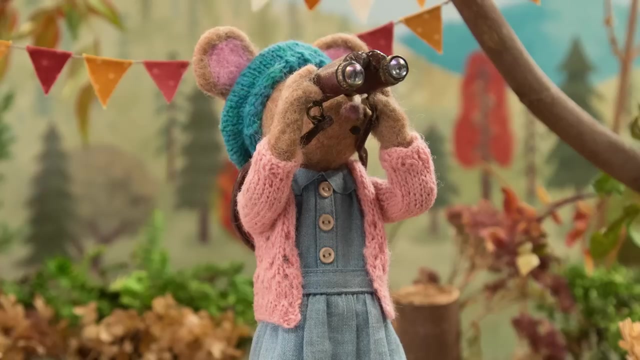 My cloud is going to be big and fluffy like this, Looking good. Great work, Gumboot Kids. Okay, step two: Let's check out a thunderstorm. Notice the shape of the lightning. Pretty cool, huh. Now let's make something cool. 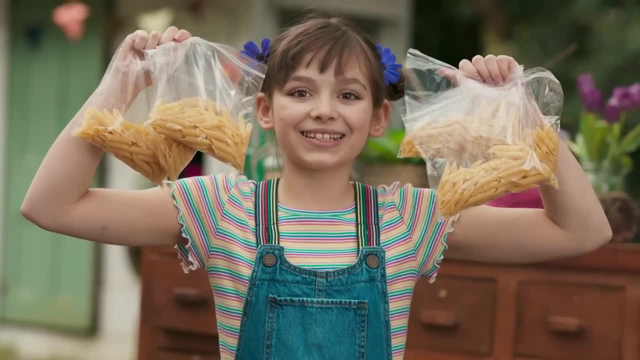 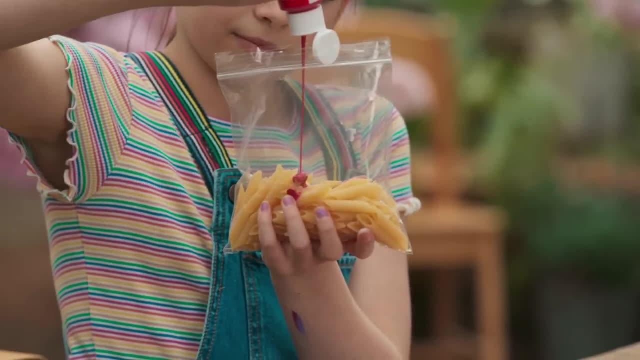 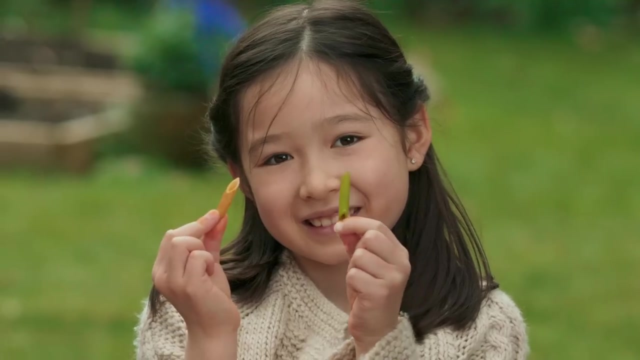 Make some lightning. Place some uncooked penne pasta noodles in a bag, Squirt some paint in and shake it up. You can create different colored noodles using different colored paint so that you have a variety of options for your lightning. After you've let the paint dry, string the penne onto some pipe cleaners. 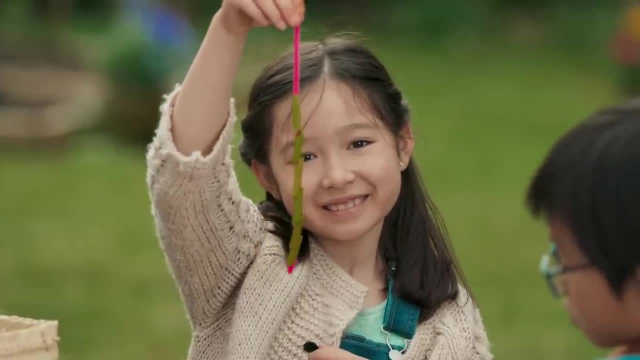 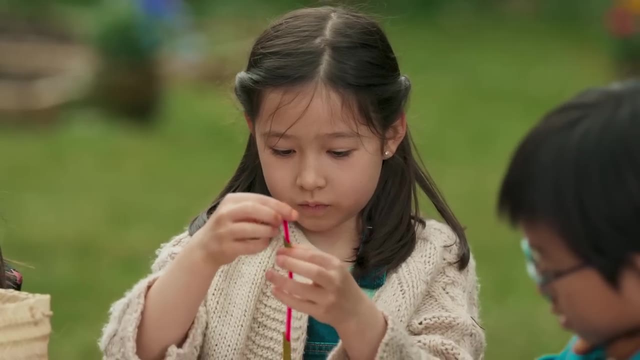 Notice how the penne creates a zigzag pattern, just like lightning. You'll need to make a string of lightning for each hole you punched into your cloud. This is fun. The pasta fits perfectly on the pipe cleaners. All right, Gumboot Kids. Now for step three. 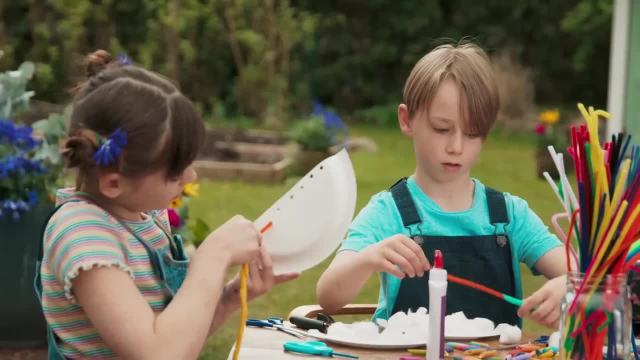 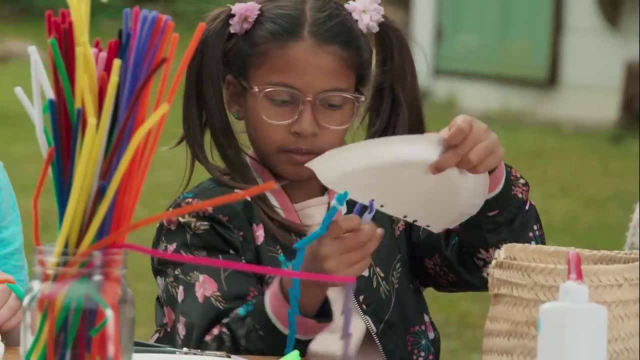 Thread your lightning bolts into the holes you punched into your cloud. Like this, That's right, Just like that. And now connect your lightning bolts to the holes. You got it All right, Gumboot Kids. Let's see what you've made.